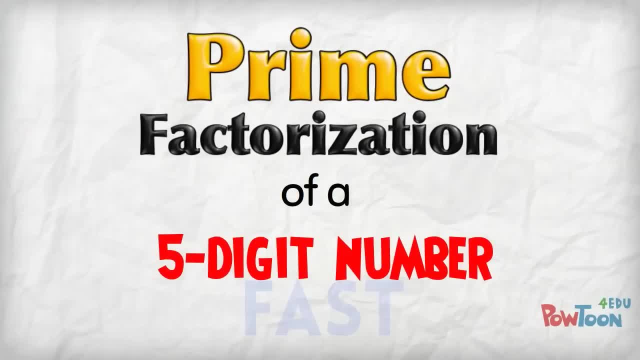 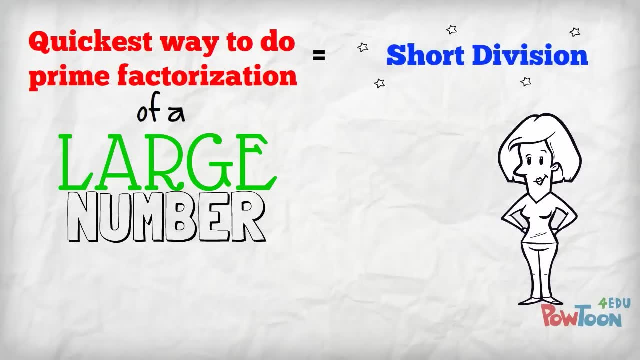 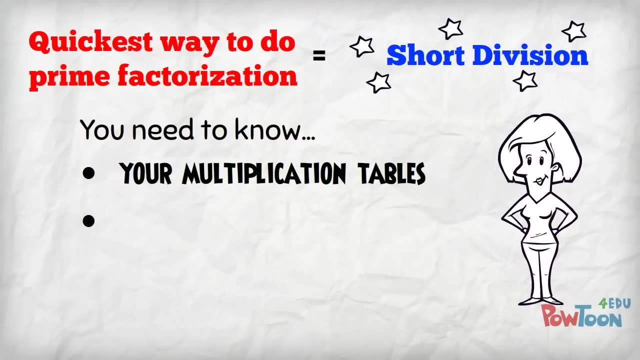 Prime factorization of a five-digit number fast. The quickest way to do the prime factorization of a large number is to use short division. To do short division you need to know your multiplication tables And for prime factorization you need to know which prime divisors to choose. 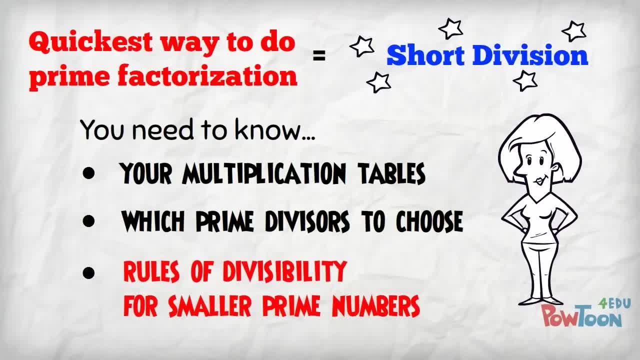 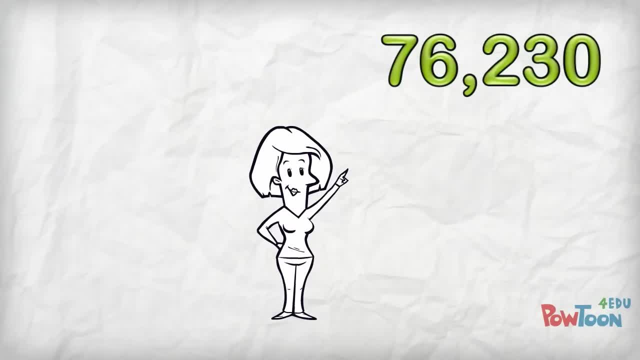 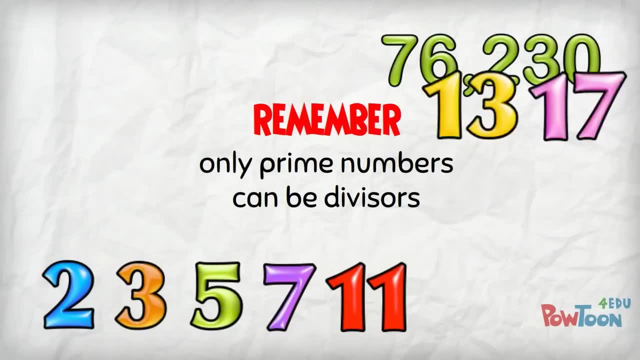 And that means knowing the rules of divisibility. for the smaller primes. I'm going to do the prime factorization of 76,230 to show how fast this method is. Remember, we can only use prime numbers as divisors And we keep on dividing until we get to the answer of 1.. 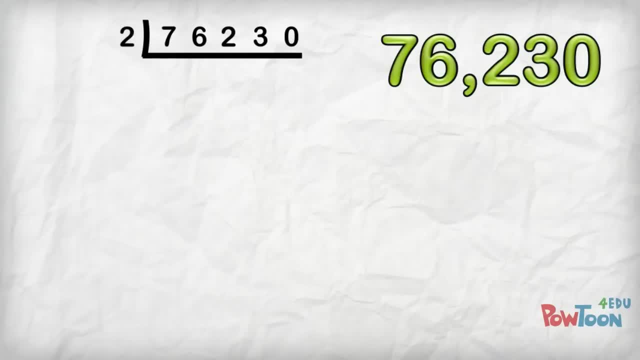 Our number is even so. I'm going to divide by 2.. 2 is into 7.. 3: twos are 6, remainder 1.. 2 is into 16.. 8 twos are 16.. 2 is into 2.. 1.. 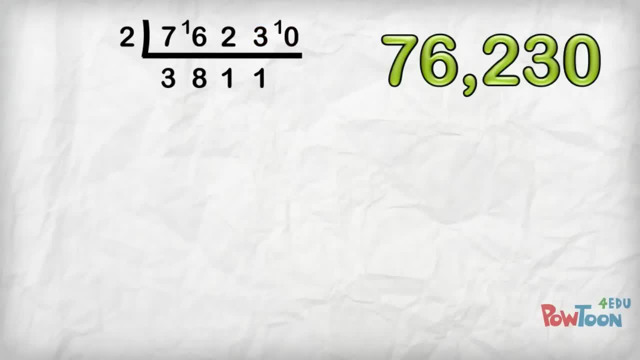 2 is into 3.. 1, remainder 1. 2 is into 10.. 5 twos are 10.. Our answer ends in 5, which means it is divisible by 5. So 5 is into 38.. 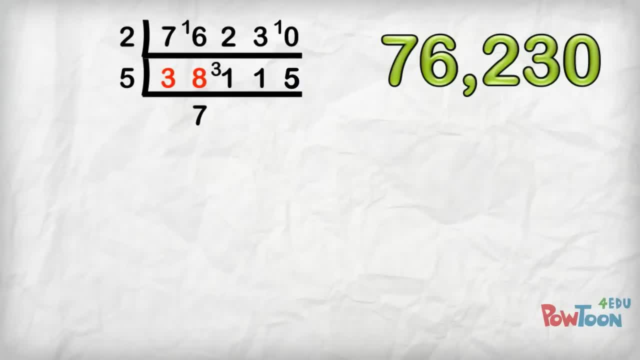 7 fives are 35, remainder 3.. 5 is into 31.. 6 fives are 30, remainder 1.. 5 is into 11.. 2 fives are 10.. Remainder 1.. 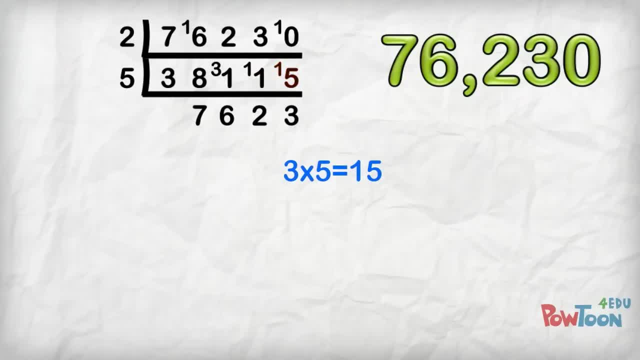 5s into 15.. 3 fives are 15.. This answer ends in 3,, so we can't divide by 2 or 5.. The divisibility rule for 3 tells us: add the digits of a number. If the total is in the 3 times table, then 3 is a factor. 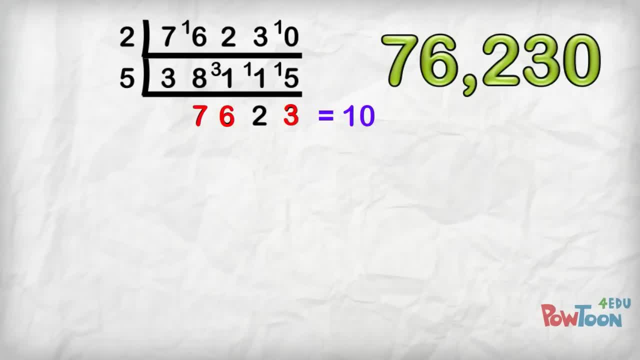 Let's try it. 7 and 3 is 10.. Plus 6 is 16.. Plus 2 is 18.. Which is in the 3 times table. so 3 is a factor 3s into 7.. 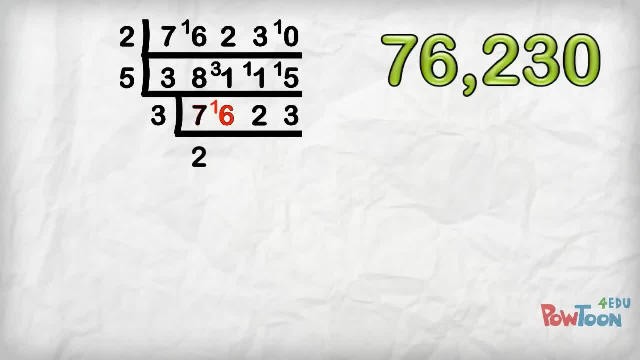 2. threes are 6. Remainder 1. 3s into 16.. 5. threes are 15. Remainder 1. 3s into 12.. 4: threes are 12. 3s into 3. 1.. 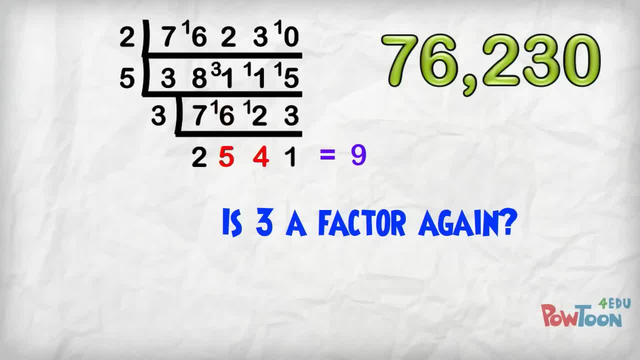 Is 3, a factor again. 5 and 4 is 9.. Plus 1 is 10.. Plus 2 is 12.. Yes, we can use 3! 3s into 25.. 8 threes are 24.. Remainder: 1.. 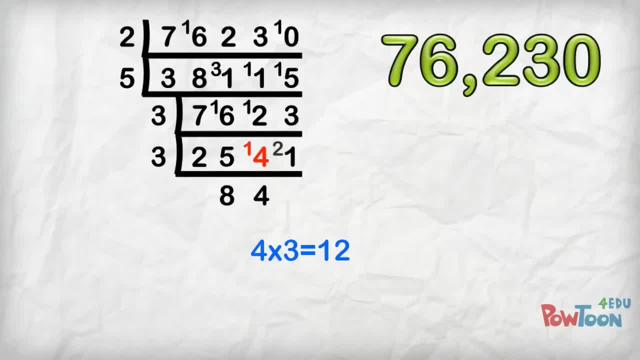 3s into 14.. 4 threes are 12.. Remainder 2. 3s into 21.. 7: threes are 21.. 8,, 4, 7.. Is 3 a factor here? 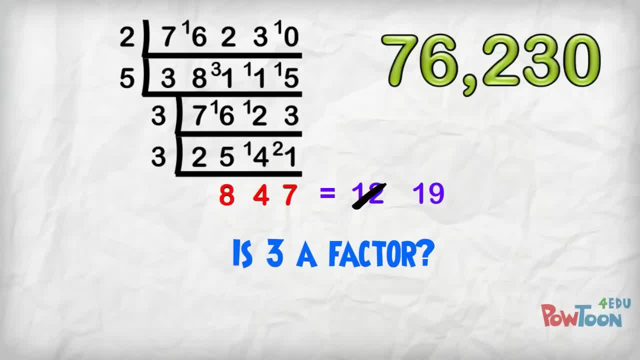 Well, 8 and 4 is 12.. Plus 7. That's 19.. So 3 is not a factor this time. What about 7?? The divisibility rule for 7 says we double the last digit, then subtract that from the value remaining. 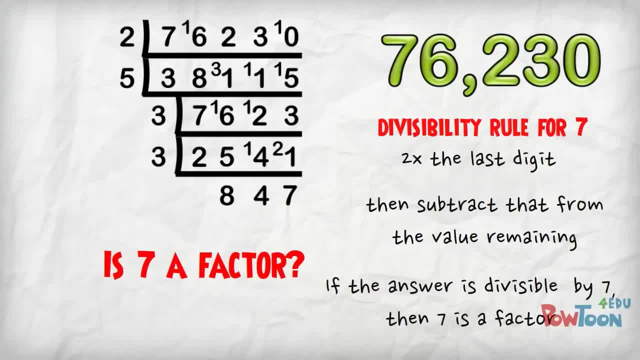 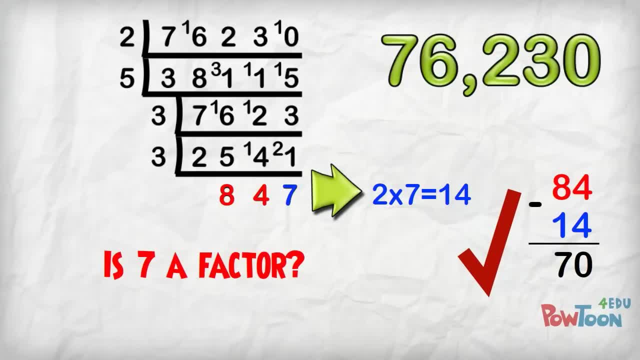 If the answer is divisible by 7, then 7 is a factor. So let's check Double: 7 is 14.. 84 minus 14 is 70.. Yes, 7 is a factor And with this number we could check just using our 7 times table knowledge. 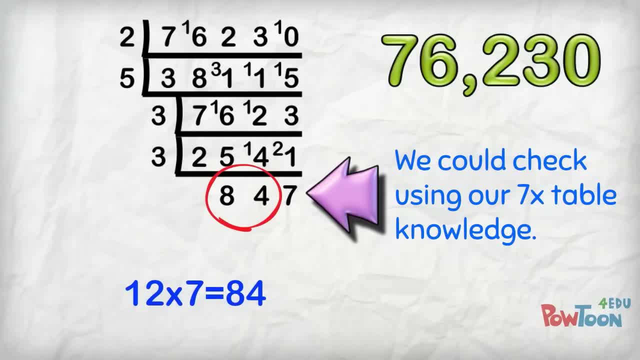 Look at this. We split the number down, We know that 12: 7s are 84. And 1: 7 is 7.. So we can see, even without using the divisibility rule, that it would work. So using short division, 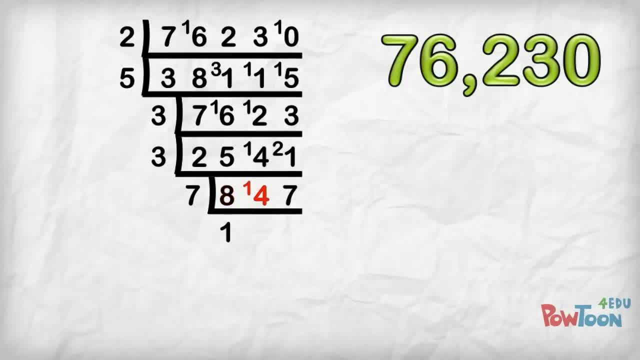 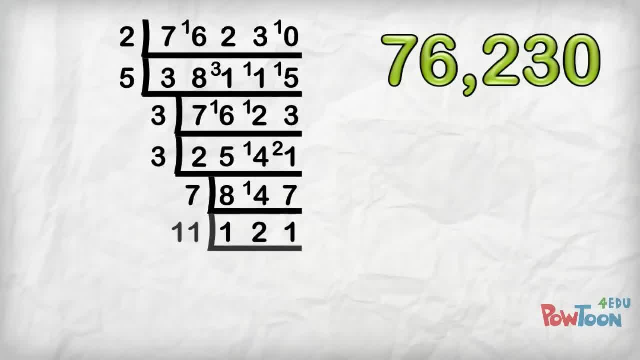 121.. I know this is in the 11 times table. 11- 11s are 121.. 11- 11s are 121. And 11 is a prime number. So 11 divided by 11 is 1.. 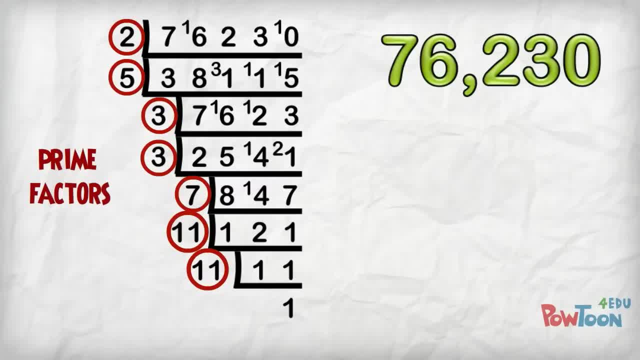 And we're done. Gather all the prime factors in ascending order. Gather all the prime factors in ascending order 2 x 3 x 3 x 5 x, 7 x, 11 x 11, And use exponential notation for the repeated factors. 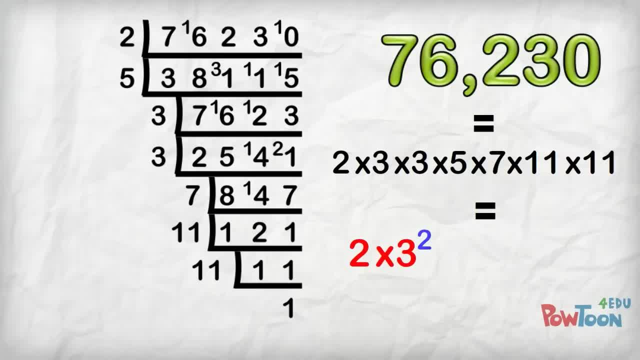 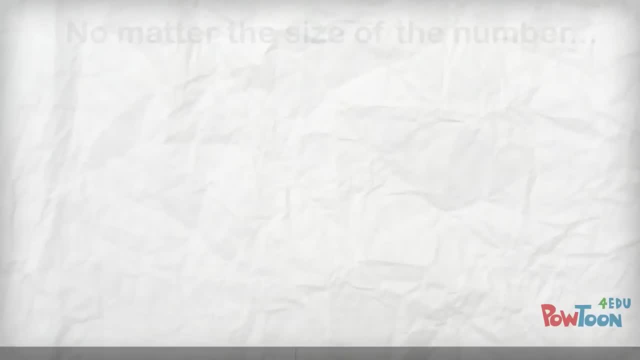 2 x 3 x 3 x 5 x 7 x 11 x 11 x 11, And we're done. That's all there is to it. So you can see, No matter the size of the number, If you know your tables.